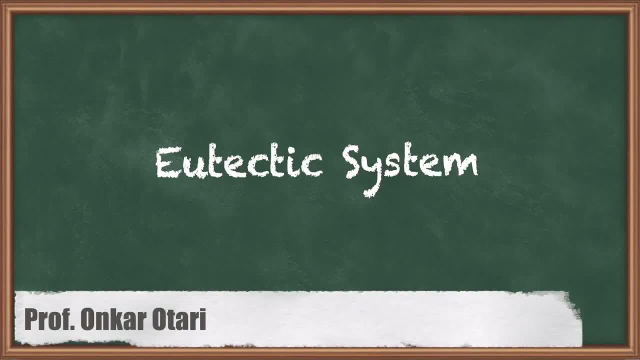 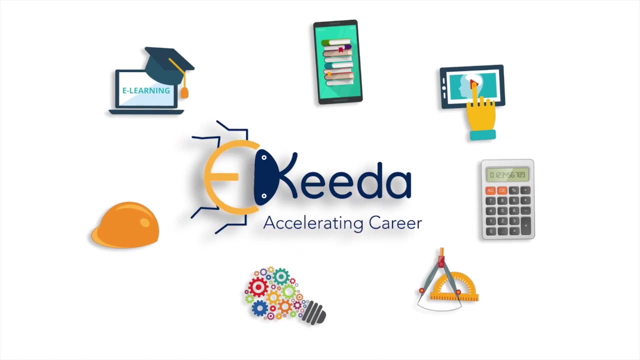 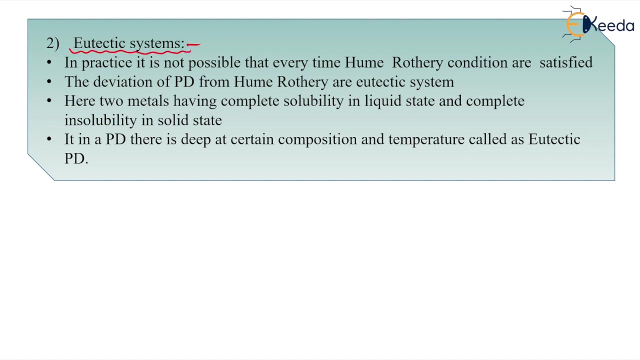 Welcome students. Now today, in this video, we are going to see the second common type of the phase diagram, that is, the eutectic systems. Here we are going to see here the eutectic system. So, dear students, we have seen the Hume-Rothri rules for the solid solubility of the two systems. 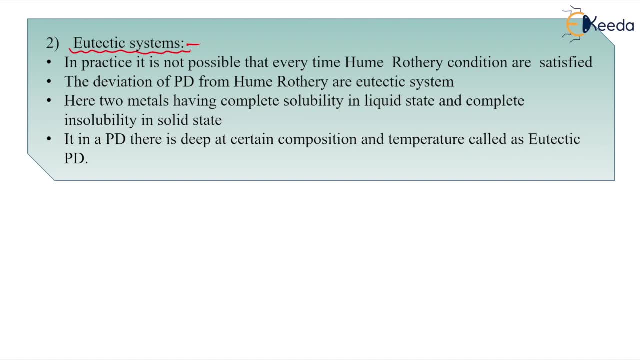 or two elements, isn't it So? but in practice it is not possible to that every time the Hume-Rothri conditions or the rules are get satisfied. So we can call it as here this eutectic system are the deviation of the phase diagrams from the Hume-Rothri? 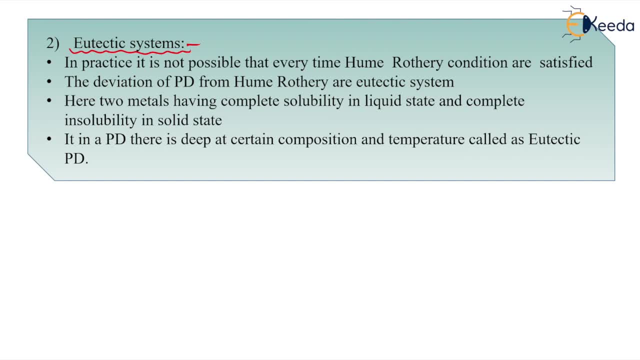 system. So we can call it as here this eutectic system, are the deviation of the phase diagrams rules. So of course we cannot able to satisfy the Hume-Rothri rules every time. So the deviation from this Hume-Rothri rule is nothing but this eutectic system. So what? 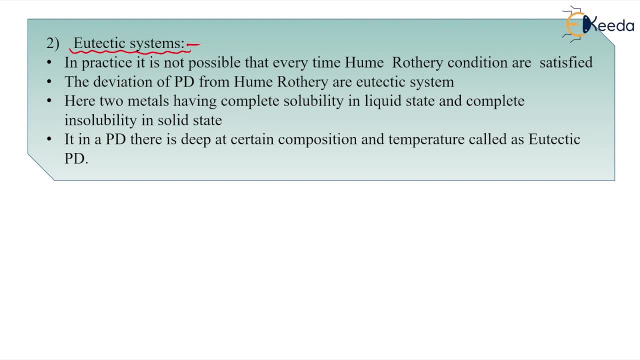 actually happening in this eutectic system. So, dear students, if you see here- this is very important- Here two metals having complete solubility in the liquid state means these two elements are having complete solubility in the liquid state. So here two metals having 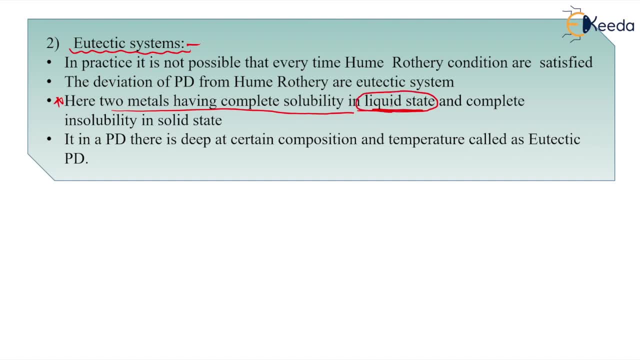 two elements are completely soluble in liquid state, but they are completely insoluble in the solid states or complete insolubility in the solid state. So this is actually the eutectic system. So what is mean by eutectic In liquid? these two elements, A and B, are completely soluble. 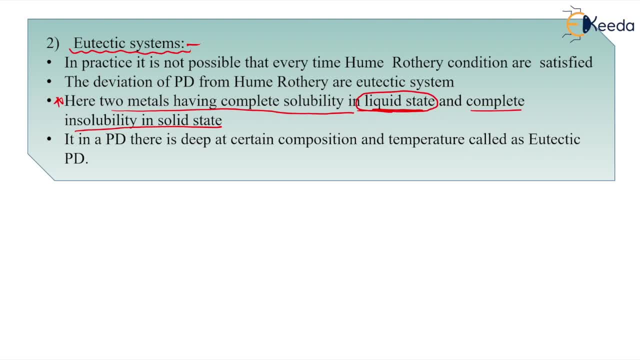 but in solid state they are insoluble. So this is the deviation from the regular Hume-Rothri conditions, that is, the solid solubility should be there, but here, in solid state, they are completely insoluble. So when you talk about, dear students, this eutectic system, So how? 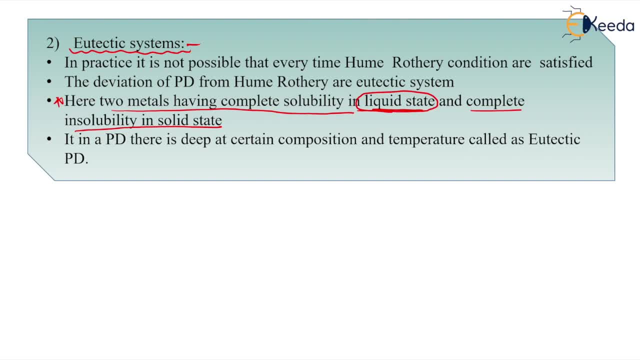 to get identify this eutectic system. So, dear students, definitely we are going to see it. but the common practice or common indication of the eutectic system is this, that is, see here if in a phase diagram there is a certain or a dip at certain composition. 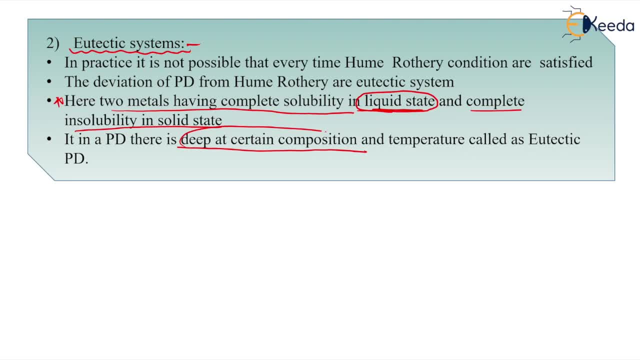 and there will be the eutectic system. Please remember, whenever there is a dip in a certain composition and temperature and temperature called it as the eutectic phase diagram. See, for example, if I have, like this phase diagram, Say this is element A and this is B, I am not showing here the solid solutions of this in 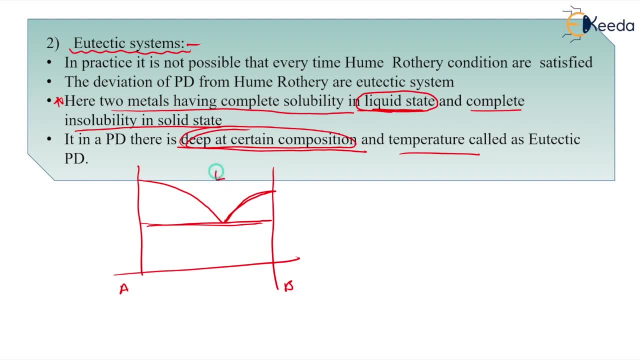 between. See like this: Say this is liquid, here temperature of A and melting temperature of B. Say, for example, like this: A plus L, B plus L, and here what we are showing, this is also locked, O, O. So are there Nu souls which are there in layered sign? So the motioning 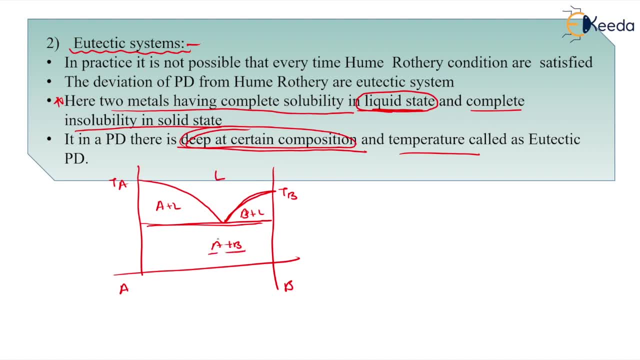 here A plus, I should write here: the phases only should be written in the Greek alphabets. that is a rule, we know that. So, dear students, you can see here: this is the melting point of element A and this is the melting point of element B, but you can see that there is a sudden dip. 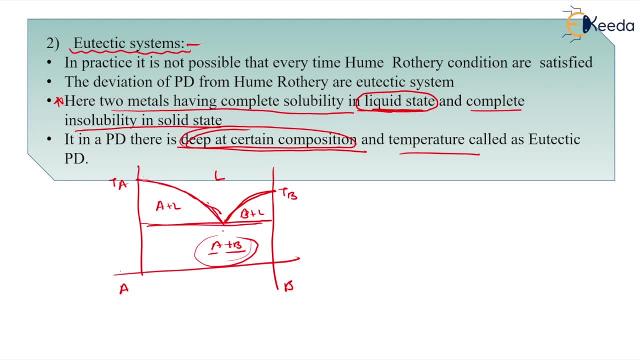 this is the sudden dip in the composition also and the temperature. So even the melting points are at such a huge distance from this point. but these two elements are meltable at this point, okay. So what is mean by actually eutectic? Eutectic is a Greek word, it means the easy. 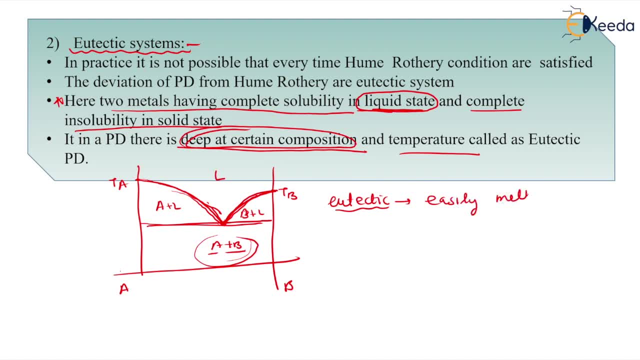 longer感じ는. elements that are not melting. So these are the easy, not considering elements that are not melting. So what is the easy? not considering elements that are not melting, So this is a meltable or nicely melting, Even though you can see here melting point of A at this point. 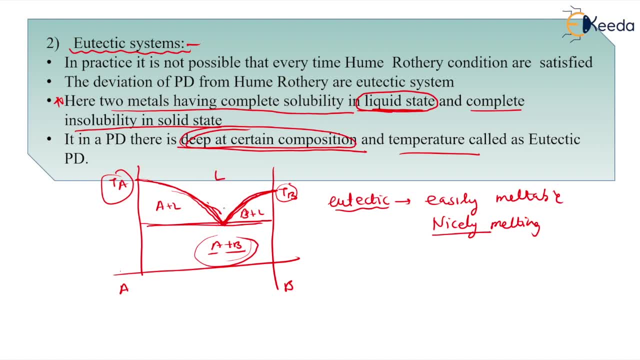 and melting point of B at that point, but both are liquid at this temperature, Isn't it? This is the eutectic temperature, Te, and the composition at this point. suppose this is percentage of x in B. So this is the eutectic composition. I will write here xE, So this: 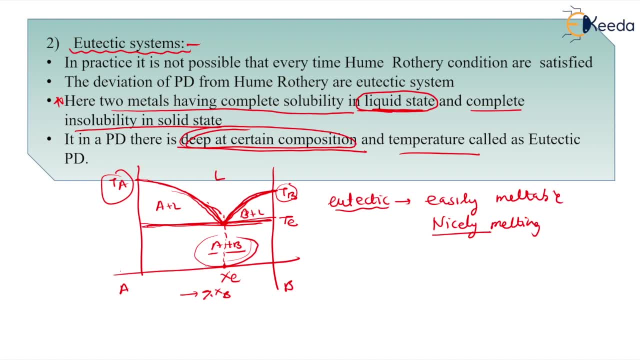 is how we can able to understand whether the system is eutectic or not. You can find here from liquid. there is a sudden dip in temperature at certain composition. So temperature is Te. Te means eutectic temperature And xE is what Eutectic composition, eutectic composition. So this is about this eutectic. 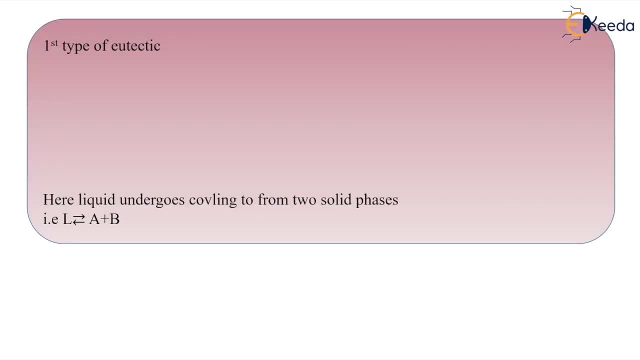 system. So, dear students, so we can have here the first type that there are the various types of the eutectic system. So the first is what? The first types, eutectic. okay, in eutectic system we are having the first type eutectic. so first, 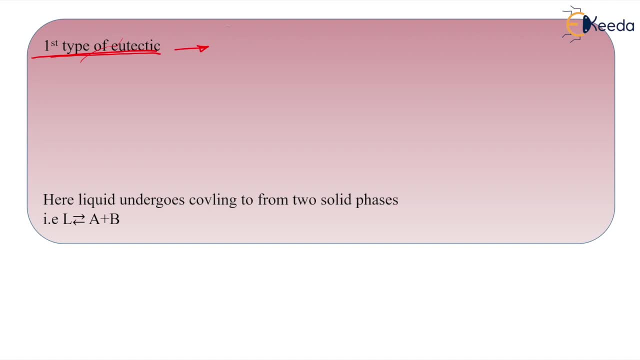 of all, if you write, want to write the reaction, what is the eutectic system? there is a certain dip you have seen here. this is a liquid and it is undergoing to form, say solid, two solids. so eutectic reaction is actually what? when you cool the material from this, it's liquid state. okay, heating or 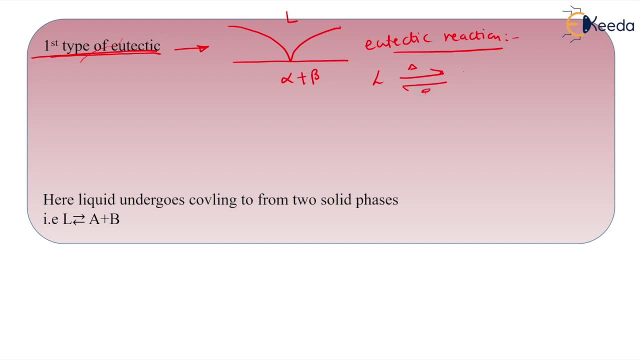 cooling, you will have the two solids I can get here: s1 plus that is our alpha phase and beta phase, say, for example, empty. so this is alpha plus liquid, this is beta plus liquid. when it cool below this Te, you will get this alpha plus beta, isn't it? 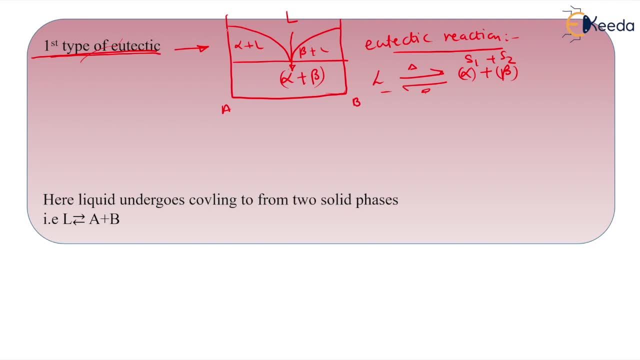 say this is element A and B, and alpha and beta are the phases in A and B. this is Ta, this is say Tb, but both are meltable at this very less temperature. that is Te as a eutectic temperature and this is the eutectic composition. and 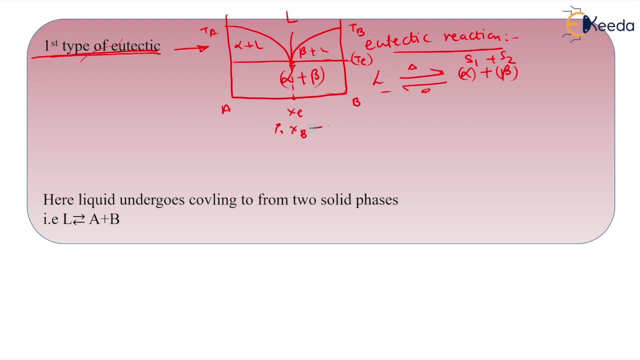 this is percentage of X in B. so, dear students, so when the liquid is undergoing cooling, it will form the two solid phases, S1 and S2. where these are, S1 is alpha and S2 is beta. so this is the eutectic reaction, and the first. 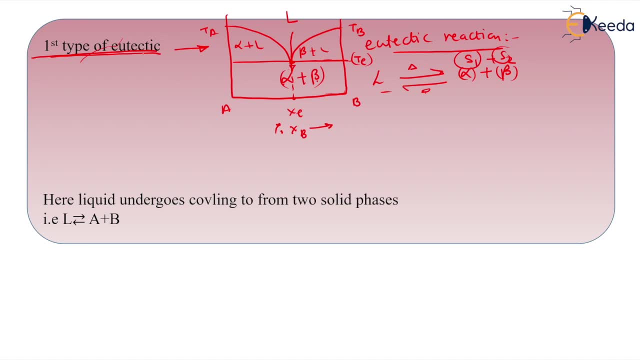 classification of the eutectic reaction is the eutectic reaction. and the first classification of the eutectic reaction is the eutectic reaction and the first classification of the eutectic system. that is, the first type eutectic system as 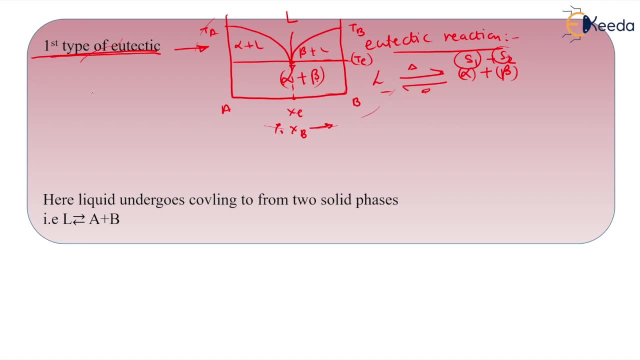 we have shown here. this diagram is for the first type, eutectic. so here we seen this reaction: liquid undergoes cooling to form the solid phases alpha and beta. okay, so when liquid cools down from high temperature to low temperature, the glow. this is reaction known as the eutectic reaction. so what is eutectic reaction? 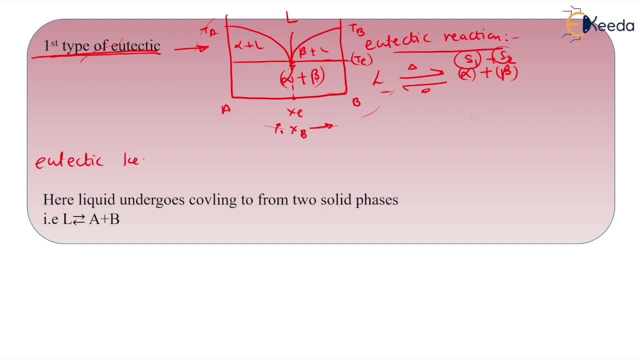 so. when liquid cools from high temperature to low temperature, this reaction is known as the eutectic reaction, and eutectic means what easy to is the eutectic reaction, when liquid cools down from high temperature to low temperature easily meltable. that is the composition. 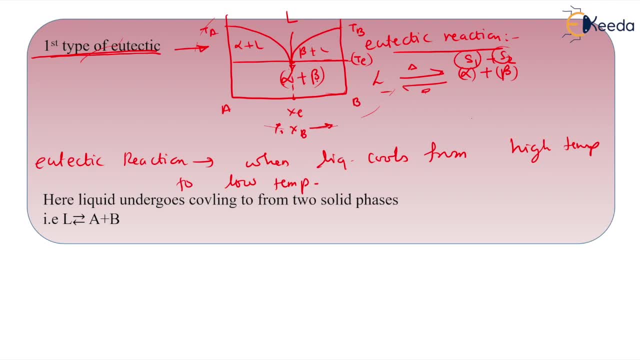 melt at low temperature, and at any other composition it is as see. if you see, at this composition only it will melt at very less temperature other than this, the temperature goes on in, isn't it? so this is the eutectic system and this is the first type eutectic diagram, so the first type eutectic diagram, we can have the examples. 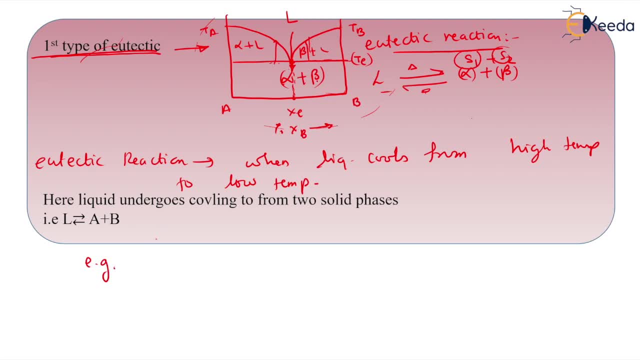 example of eutectic diagram. we can have the example of the first type eutectic diagram. we are having the lead and arsenic, we are having bismuth and cadmium, we are having the thorium, titanium and this gold and silver. so these are the elements. 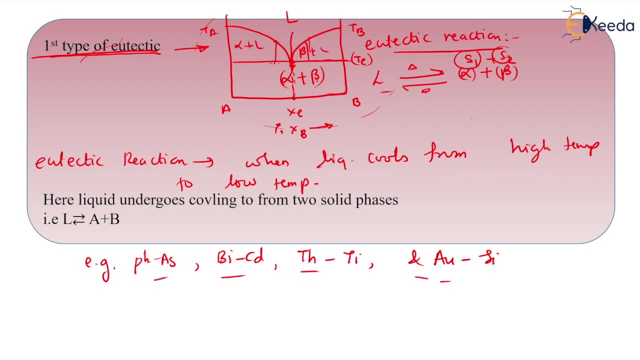 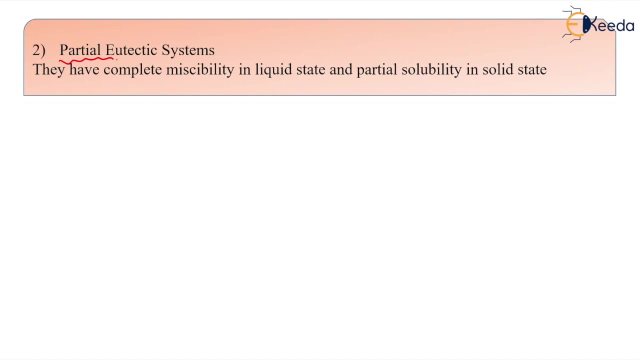 or phase diagrams which are having this first type eutectic system, then the second we already seen here. the second type of eutectic system is known as the partial eutectic system, dear students, the second type of eutectic, that is the deviation. 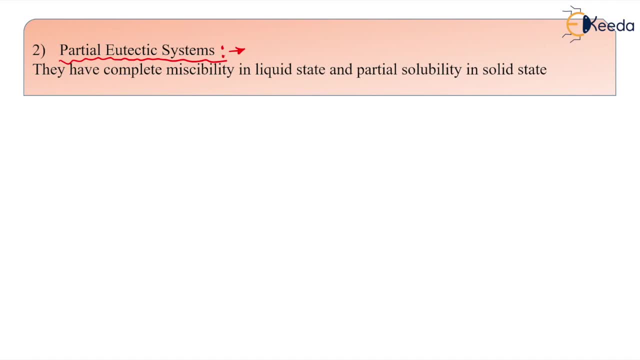 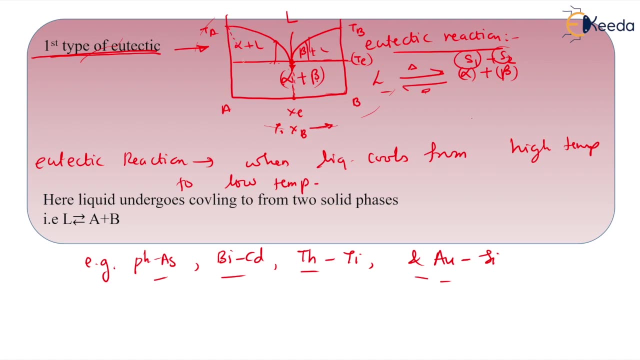 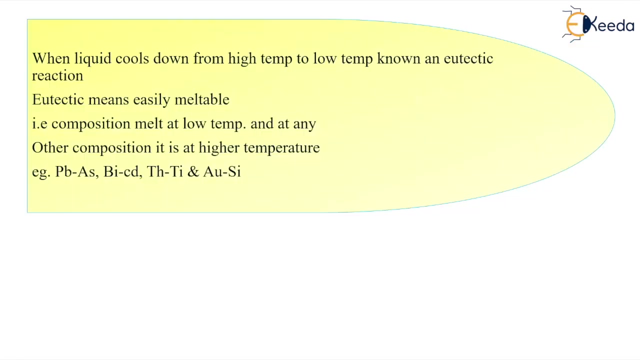 from the humul three rule. first, we have seen this is the first type eutectic. so the thing is that, dear students here you cannot see here the presence of eutectic号, of the solid solution of A and the solid solution of B. But yes, when we are saying this, partial, 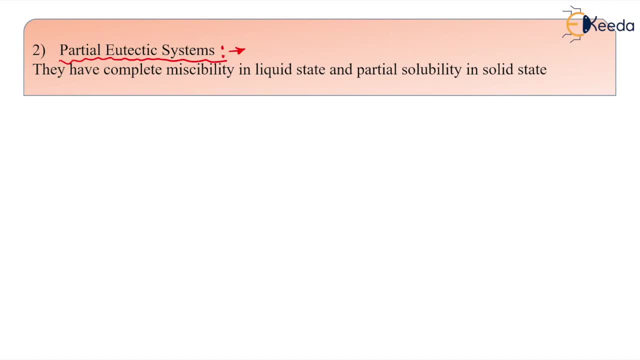 eutectic system. so we will find here the presence of these solid solutions. So what is mean by actually this partially or partial eutectic system? So here these two elements have the miscibility in the liquid state and partial solubility in solid state Means. 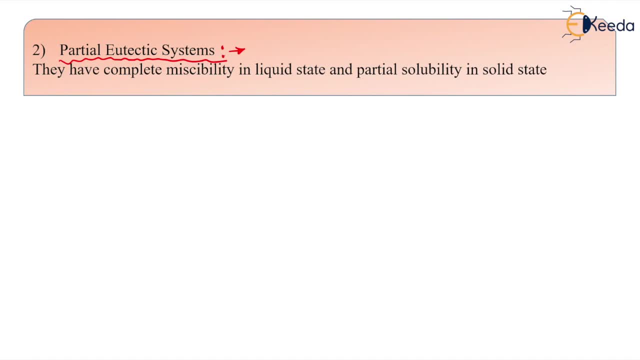 in. if you say in liquid they are completely miscible, but in solid state they are partial somewhat, they are soluble. So this is the partial eutectic system. we have written the definition here. They have completely miscibility in the liquid state, but partial solubility. 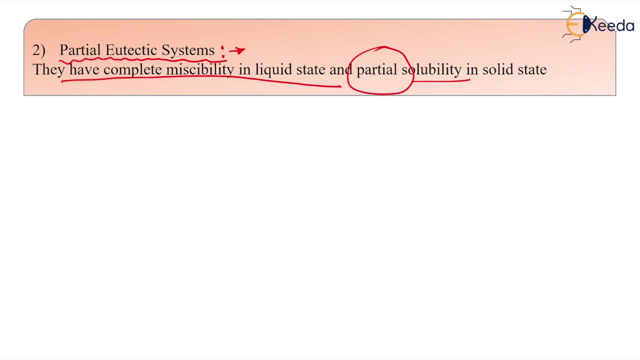 in solid. So this is the partial eutectic system, the second kind of the eutectic system. So, dear students, if you look at the very famous diagram for this partial eutectic system, so that will be lead and tin very popular. This is the classical eutectic system. So see here. 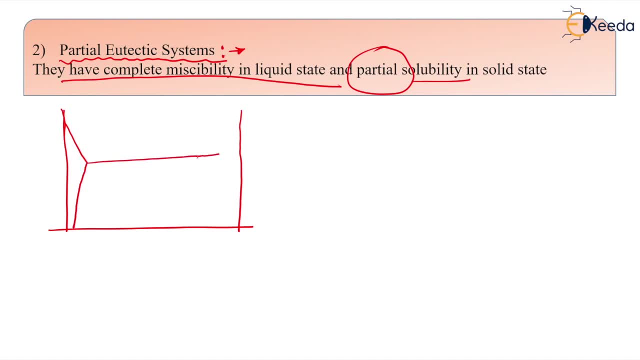 I am drawing it: lead and tin Tin phase diagram. Ok, but I will not write the name directly. So a, b. we have seen element. I will take here d and e. So this liquid and suppose alpha is the. 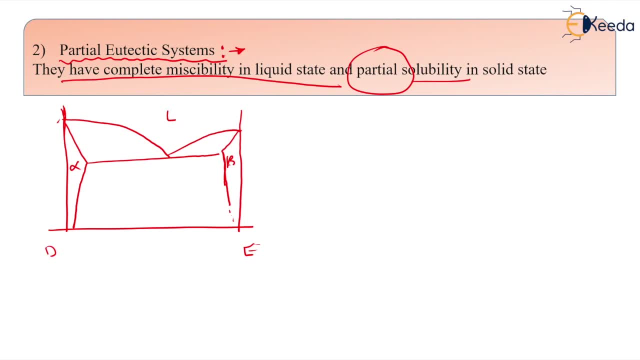 phase in d, solid solution. beta is the solution of e- alpha plus liquid, beta plus liquid and e is individual. Yeah, we have seen lead Superb. right, this is the eutectic point, this is the eutectic temperature. say this is x in e. 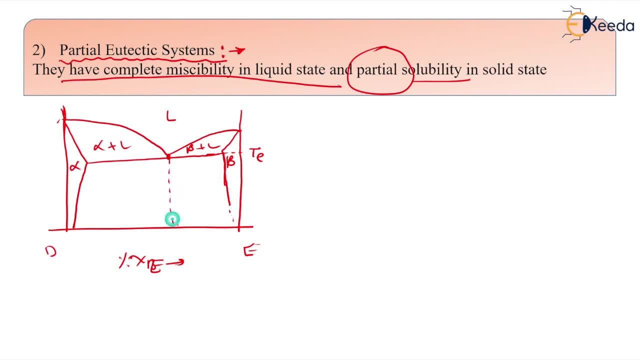 percentage, the composition here, the eutectic composition: x, e. okay, so here, see here the phases alpha plus beta, below this eutectic line. this is temperature of d, melting point of d, this is melting point of capital e. so, dear students, see here, you can see the sudden dip in a. 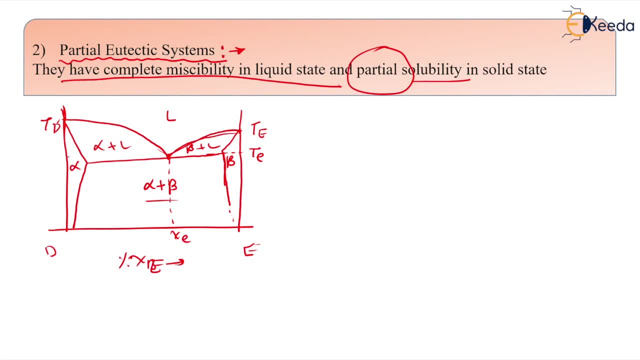 temperature at certain composition. but only the thing is that from the first type eutectic you can see the difference. here they are having the solid solution here, isn't it, of d, and the solid solution of d. okay, so this is actually the partial eutectic system, isn't it so here you can see here the two parts. one is at d, d rich. 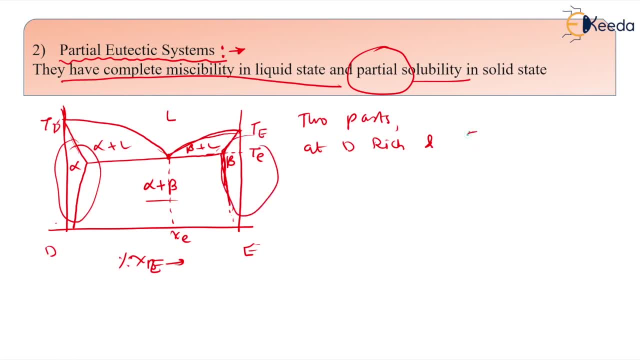 and this is the d rich region and this is the e rich region. having these solutions, alpha and beta, isn't it? and the eutectic reaction is that it is. see here, liquid undergoes cooling to form two solids. that is, liquid undergoing cooling or, again, reverse heating. you will get these two solids. 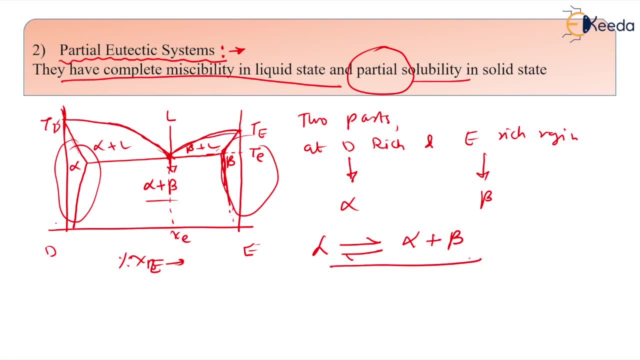 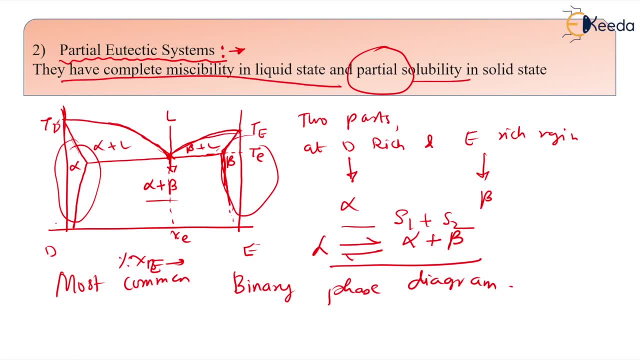 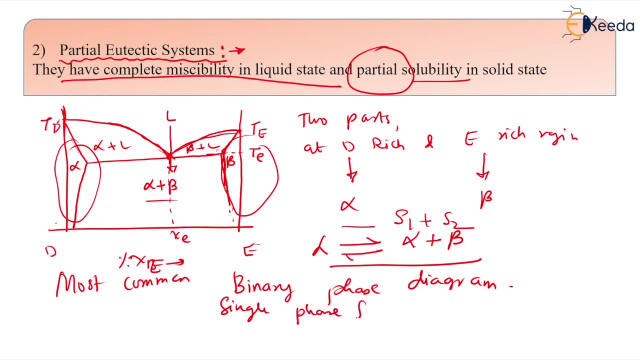 this is the most common eutectic reaction. this is the most common eutectic reaction. single phases- alpha, beta and liquid. So three single phases- alpha, beta and liquid- and two phase fields or double phase fields. how many are there? See, here this is alpha. 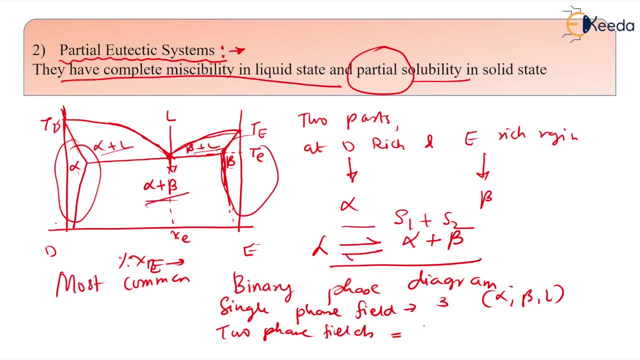 plus liquid, beta plus liquid and alpha plus beta. So there are again three. two phase fields are there, So, and you can see the number of reactions in the diagram is how many. So the rule says that we know that in the phase diagram, every horizontal line 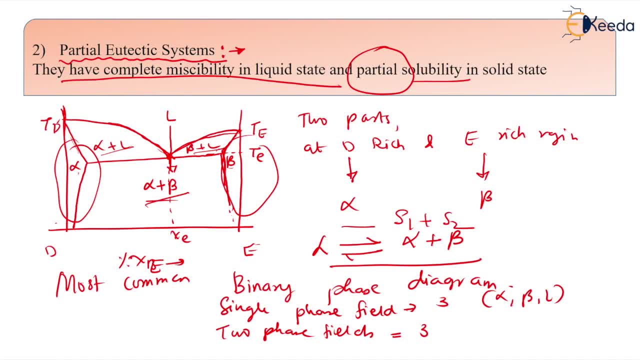 every horizontal line in the phase diagram. it is not the line which is drawn by we peoples, this is the actual. the line, horizontal line which is present in the phase diagram, will give us the one reaction. So see, here, one horizontal line is there. see, this is a horizontal. 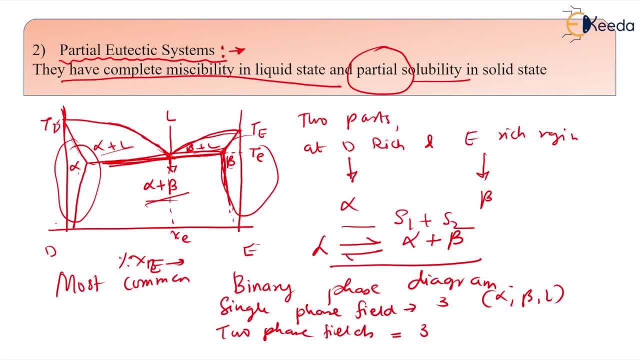 line and this line is giving this the reaction. what? What is the reaction? So liquid undergoes cooling to form alpha plus beta. So see here, here, liquid is slowly transforming into the solids and these solids definitely going to give us the different microstructures, dear students. So, whatever the evolution of microstructures, 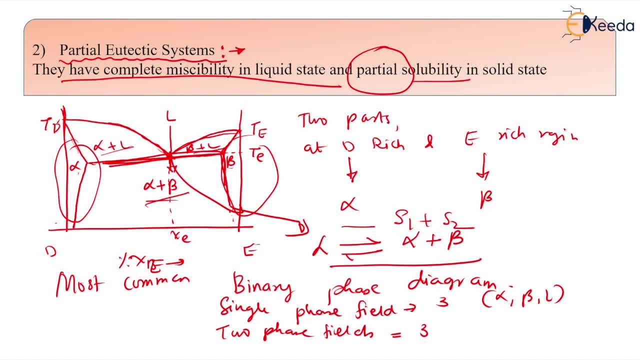 in the respective phase systems, in the phase diagrams. we definitely we are going to see it one by one. So this is the one reaction, So this is the one reaction, So this is the one, And therefore the basic point is to be stressed, that for the reaction we have, 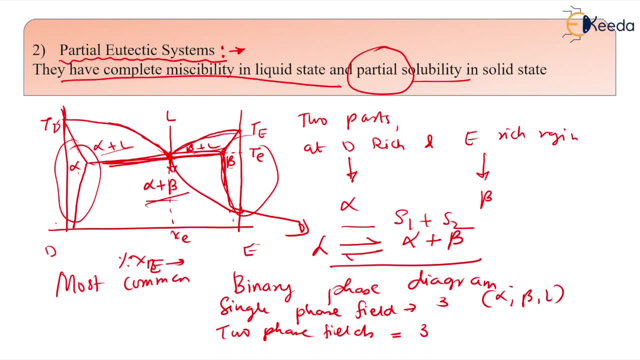 large amount of microstructures developed here. So for this reaction: definitely we are having large amount of microstructures that are going to evolve and we are going to see it in that great details. Now, because of see this, we are going to have various microstructures, but in the type 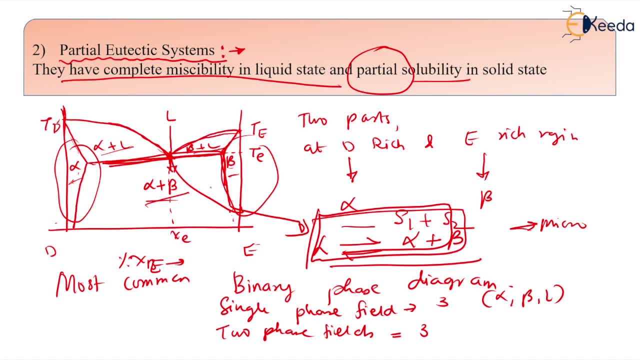 1, as this D-rich and E-rich, we are having here the solid solution In first type. we didn't found it, So that is why this microstructure also are not there in the first type. So, dear students, if I take this classical example of 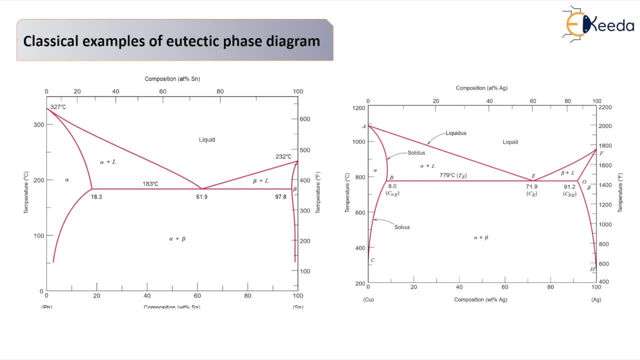 So, dear students, if we see this, one of the classical example of this eutectic phase diagram, So this is our lead and tin alloy used to make the. This is lead and tin alloy which is used to make the shoulders. So this is actually, dear students, the classical, classical. 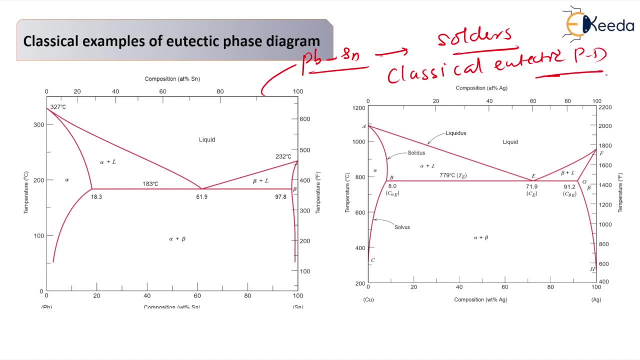 eutectic phase diagram: See this lead and tin. So we have here, we are having here this lead and tin. This is the lead here at left and the tin at the right. The melting point of the lead we are having it is 327 degree centigrade, whereas tin it is 231.9.. 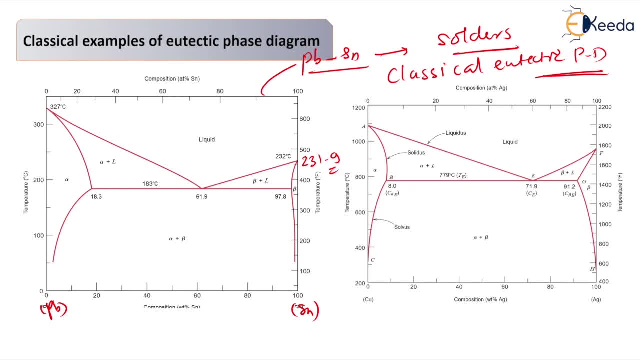 Isn't it? Yes, This is the lead that is here, 232, shown. So you can see, here the solid solution of lead is alpha and tin is beta And here is at temperature you can have here to around 183 degree centigrade. 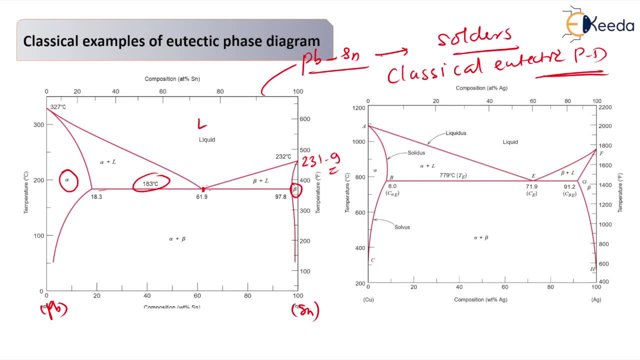 This is 183 degree centigrade line. This is one line horizontal line definitely give us one reaction that is: liquid undergoes cooling to form alpha plus beta, These two solids. This is the eutectic reaction, This is the eutectic composition here. Xe eutectic composition. 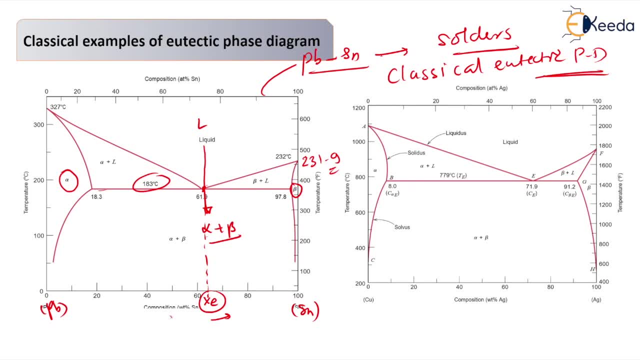 here and that is percentage of here, what Tin. And if you see here this composition is how much: 61.9 percentage of tin, Yes, Yes. So here these two elements, that is, lead and tin, one is having the melting temperature. 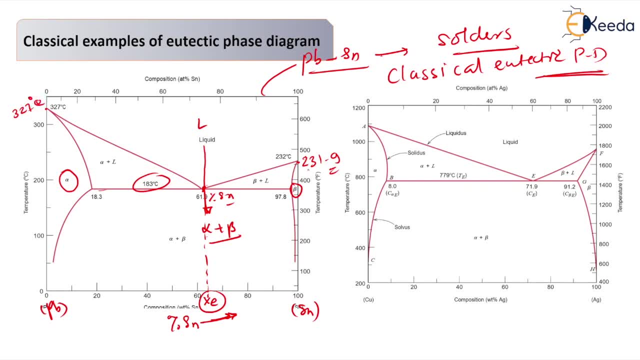 327 degree centigrade, other is having 232 degree centigrade, But these both are meltable at such a low temperature, that is, at 183 degree centigrade. That is the eutectic system, Isn't it? 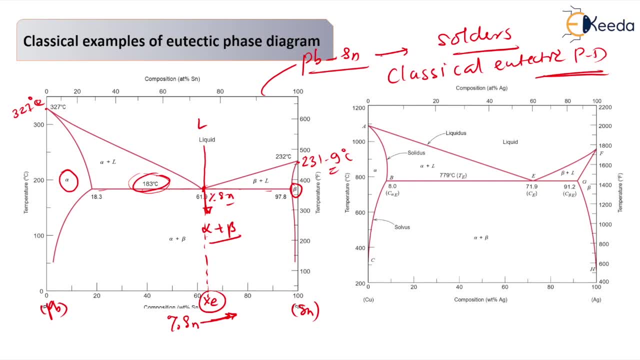 Yes. So we have to, we have to interpret this diagram. We can find here: how many single phase fields are there? So single phase fields, how many there This liquid, alpha, beta. So three single phase fields, two phase fields. Again we are having alpha plus liquid, beta plus liquid. 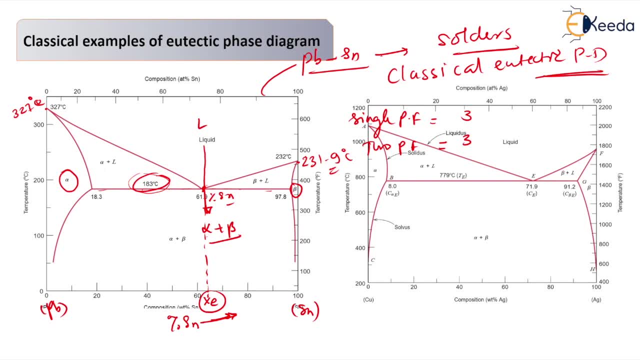 and alpha plus beta three. So, dear students, if you go on interpreting this diagram, and- and we are trying to apply this phase rule at this point, that is eutectic point- say E as our eutectic point. So, at the eutectic point, what is our phase rule? condensate of phase rule. 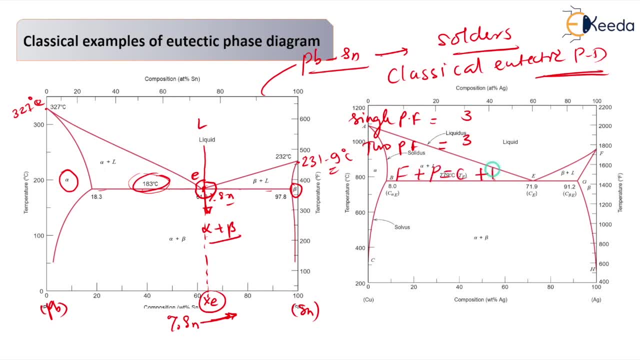 F plus P is equal to C plus 1.. Why I am taking here 1? because pressure. I am assuming that it is the constant for every reaction that is atmospheric pressure is there, So the variable is 1, only that is the temperature. So, dear students, come to this. 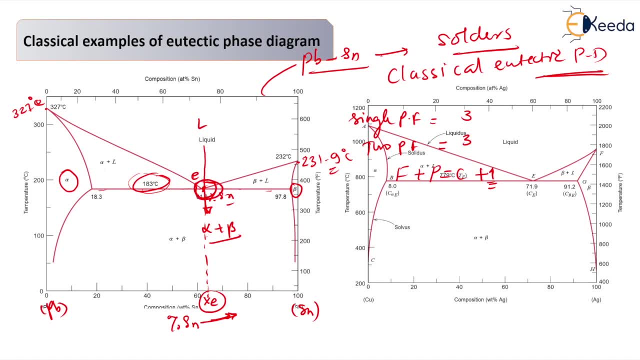 point E, that is our eutectic point, and apply this phase rule. So for that we are going to find out this degree of freedom. So how many phases are there? There are three phases: liquid, alpha and beta. So three phases are there. Components are there- this is binary system, lead and tin. How many? 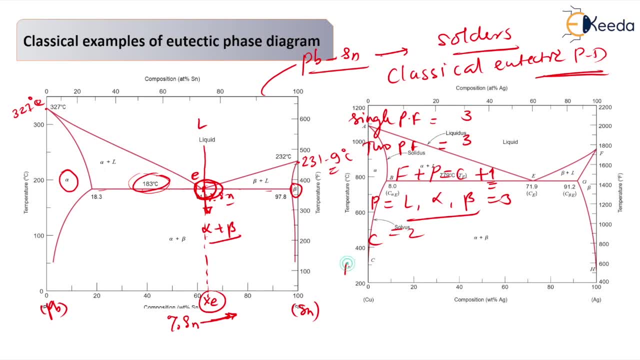 components, Two components. So apply the phase rule and find out the degree of freedom. So we are going to find out the degree of freedom. So we are going to find out the degree of freedom. F plus P3 is equal to, C is 2 plus 1.. So how much the degree of freedom? 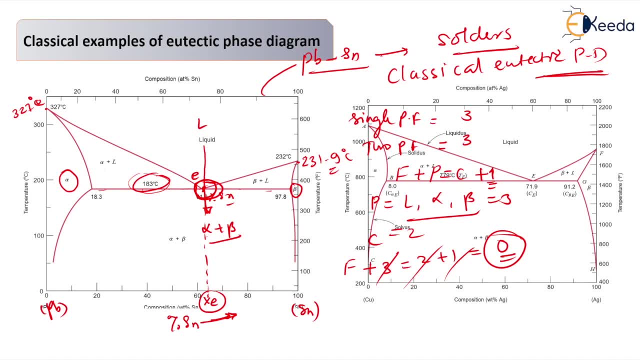 at point E that, or at eutectic point, is definitely almost 0.. So, dear students, what is mean by the degree of freedom 0 in the phase diagram? that is, that point E is called as the invariant point. The invariant, that is what you cannot able to vary, that point. 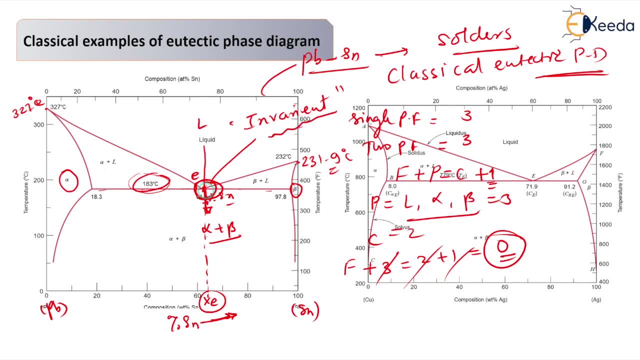 As soon as you go just below that point, you will be out of that compositions here. you go to the left, you go to the right, you go below, or you go below that point. you will be thrown out of that composition immediately. you will know more at that point if you go above. 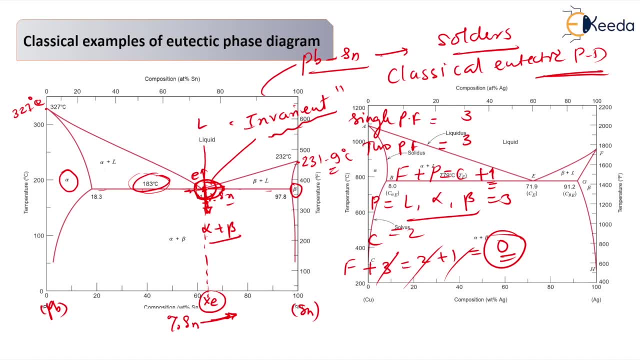 you will be liquid in, you go below. you have two solid phases, So like that you cannot able to move from that point. So you are get restricted, so that point doesn't have singularity. So the point dessarpline, may bold be. 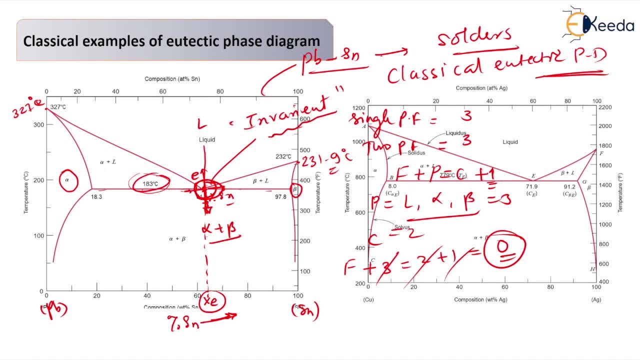 is known as the invariant point, Dear students, please remember, in the phase diagrams- this is applicable for all phase diagrams- where the degree of freedom you get 0, that is the point- is known as invariant point. So we cannot vary both the temperature and composition, and still we are. 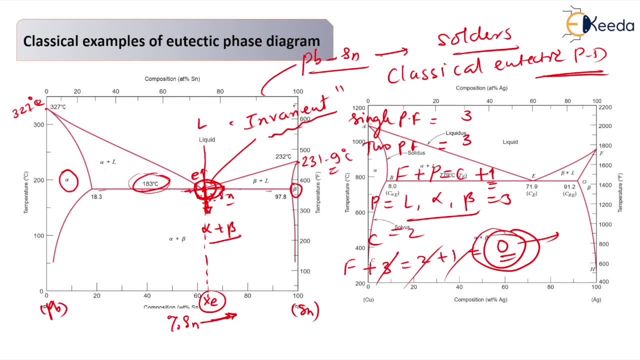 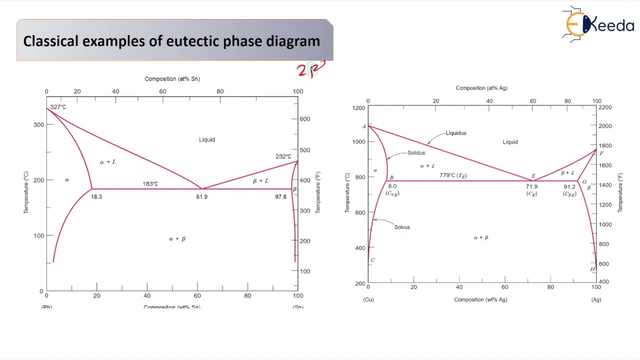 having in the same phase field. Suppose if I consider the two phase field is considered like this: this alpha and beta or this alpha plus liquid, So what we can have phases, how many phases for two phase fields? If any of the phase field, let us say alpha plus. 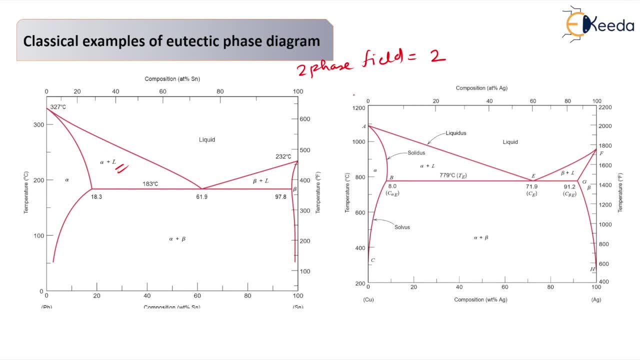 liquid. How many phases are there? Two phases are there. Components kitne hai Ladent in two components hai and apply the phase rule. F plus P is equal to C plus 1.. So F plus P is how much 2 is equal to. 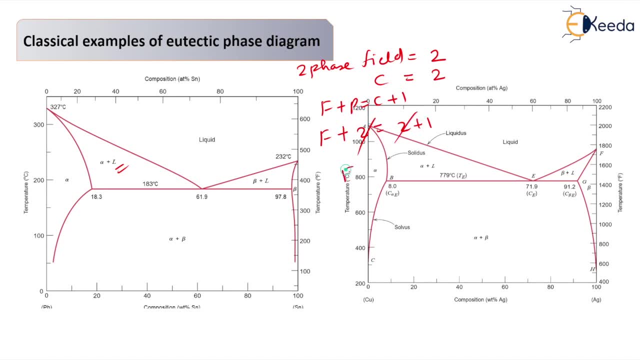 C2 plus 1.. So 2 to get cancelled, F is equal to 1.. So what is this? The degree of freedom is 1, isn't it The degree of freedom 1.. So what is meaning of this? So degree of freedom 1 is known as actually the univariant point.